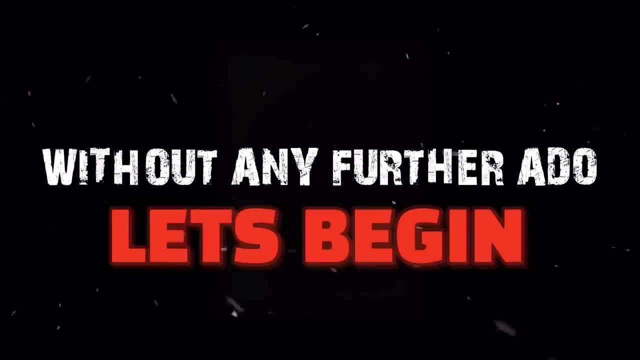 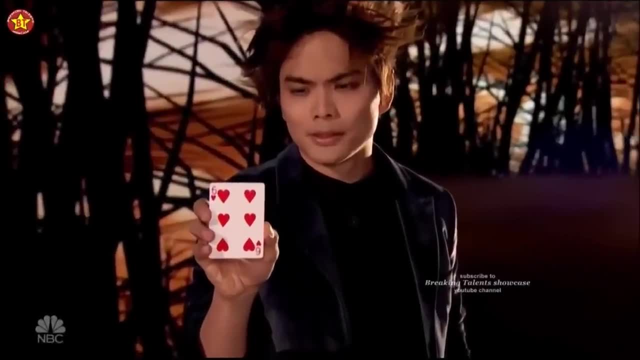 viral tricks. Without any further ado, let's begin Shin Lim's Wicked Sorcery. Let's do a quick recap of what happened in the performance. In Shin's trick, he picks a six of hearts playing card at the table and transforms it visually into 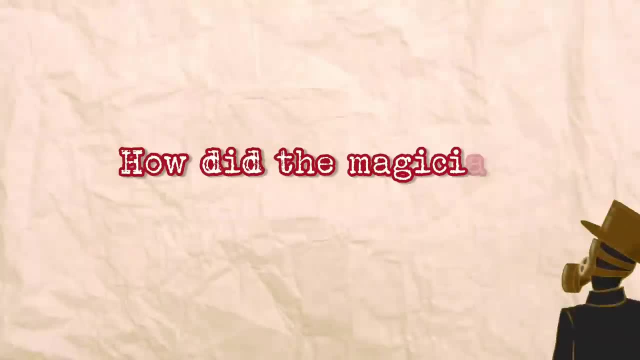 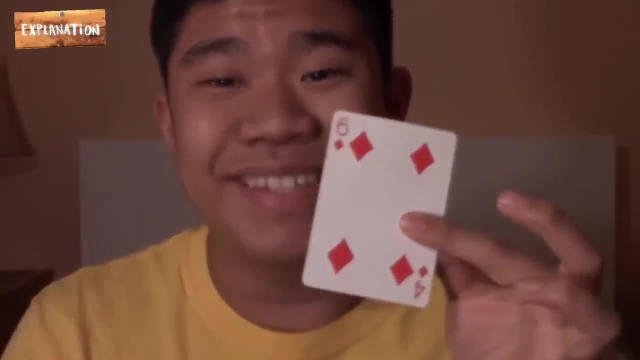 a nine of hearts card, as if it was CGI. How did the magician perform his illusions? Here is how he did it. Shin begins his illusion by covering one of the pips on the card with his hand. Then his finger is placed on an extra card piece on the back of the card, which he slides back and forth. 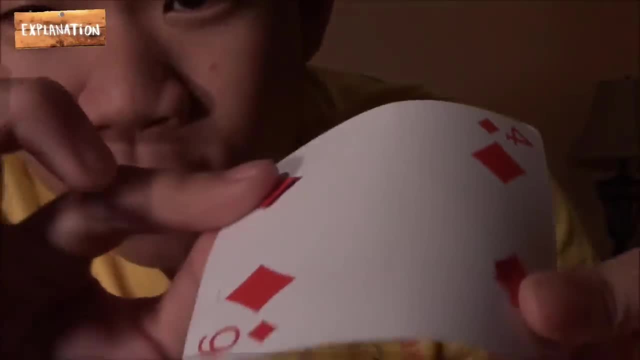 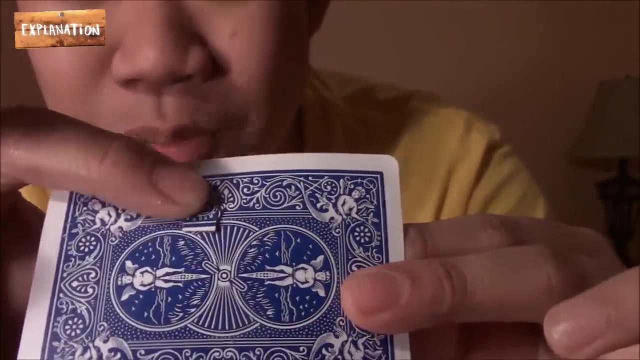 This piece of card is connected with an invisible elastic string to the movable pips on the card. Also, the extra card piece is of the same pattern as the back of the card, so it is well camouflaged and is unnoticeable. 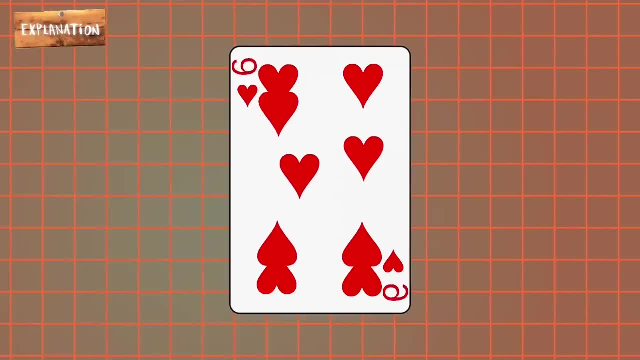 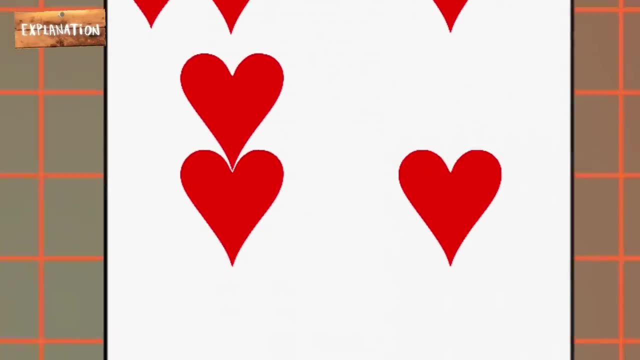 As he slides the extra card piece with his finger, it moves the movable pips and increases the number of hearts on the card. The pip on the top left corner is overlaid, so the laid pip moves downward. Also, the pip on the left side of the middle row moves to the center. Similarly. 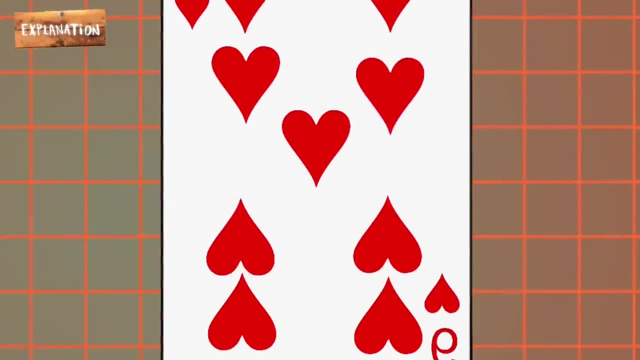 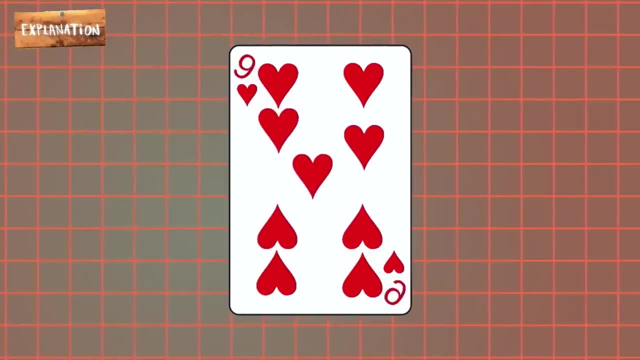 the pips on the bottom row and the pip on the right side of the middle row are overlapped, so the laid pips move upward. To make his trick seem like real magic, Shin shakes the card while moving the pip. Each of these pips moves at the same time because five strings are connected to. 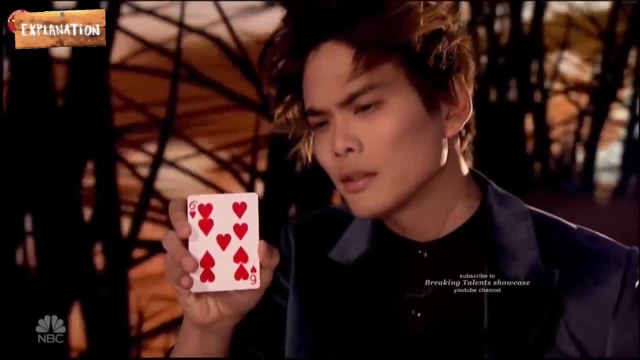 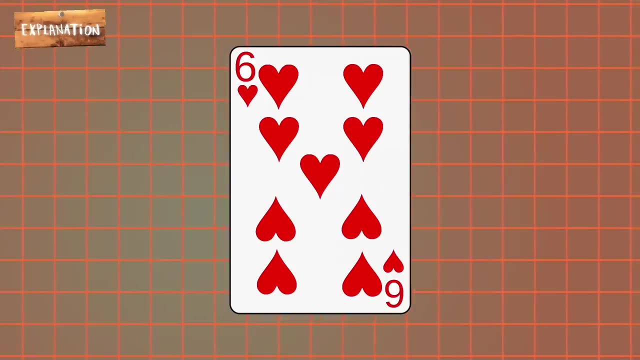 them in a straight line. Additionally, the numbers on the card are not printed on it, but are removable oval-shaped cutouts that have invisible threads connected to them. To make his trick work, the magician pulls the invisible threads from behind the card, like he. 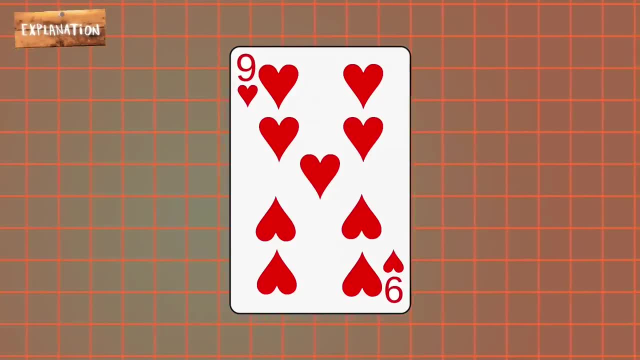 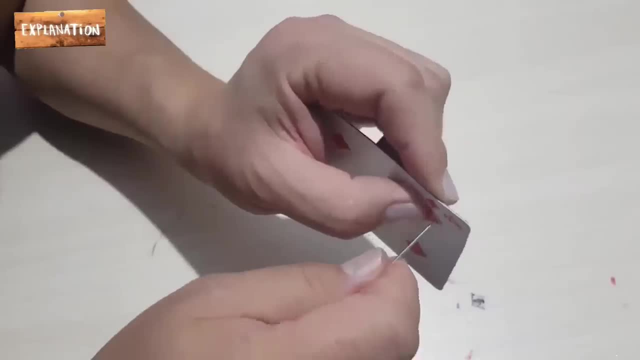 did with the pips, Then the six changes to nine by turning 180 degrees. Furthermore, a needle and the aforementioned invisible string were used to sew the pips and numbers to the card. The aforesaid piece of card was also sewn to the back of the card using the invisible thread and a needle. 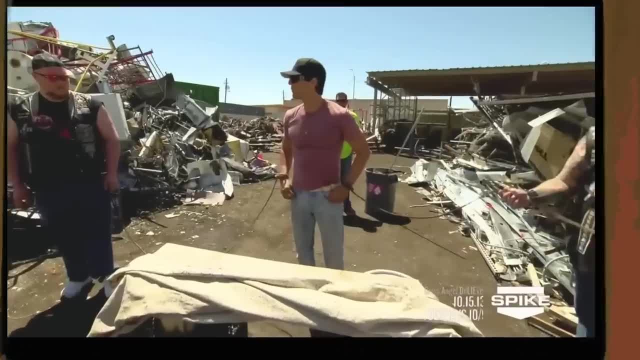 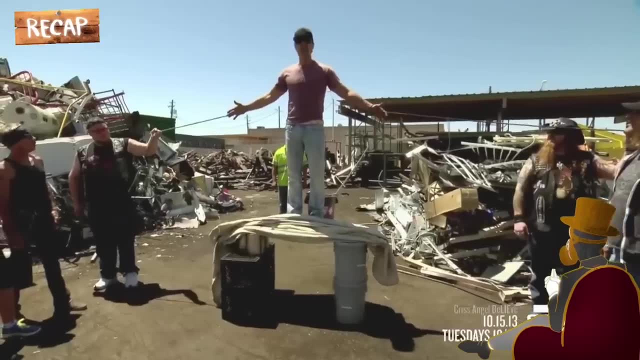 The Vanishing Criss Angel. Let's do a quick recap of what happened in the performance. In this trick, Criss climbs a slab that is placed on two supports on both ends. Two ropes are tied to both of his hands separately and pulled sideways While he stood on the slab. 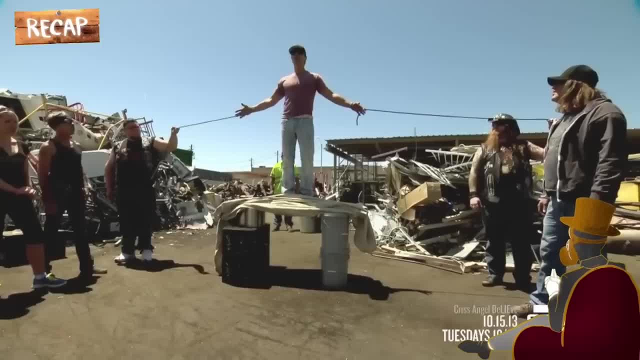 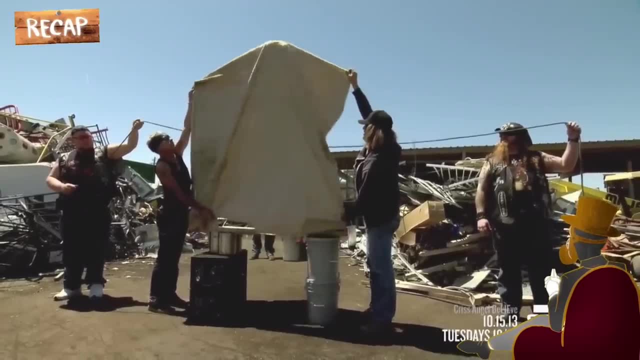 with his hands being pulled sideways. there was nothing below, above or around him. Thereafter, a curtain is used to cover him from his shoulders downwards. Suddenly, the curtain is dropped, he vanishes into thin air and the ropes appear to be tied together. 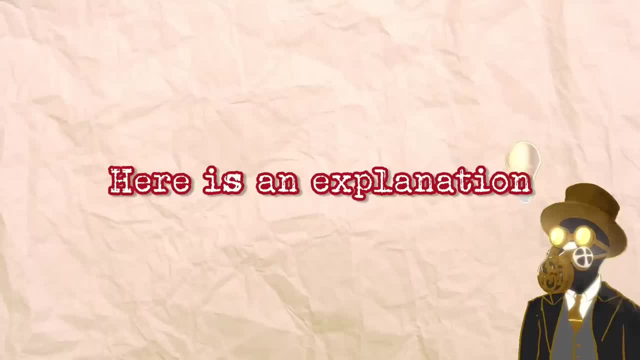 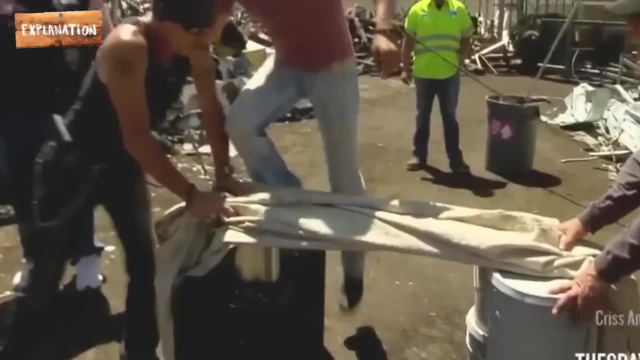 Wondering how Criss executes his illusions. Here is an explanation. At the beginning of his trick, when he climbs the slab, we notice every one of his assistants had a shadow. Similarly, the man behind the magician wearing a fluorescent yellow shirt and the barrel. 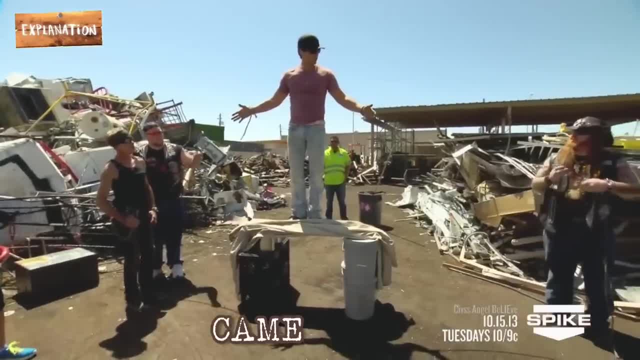 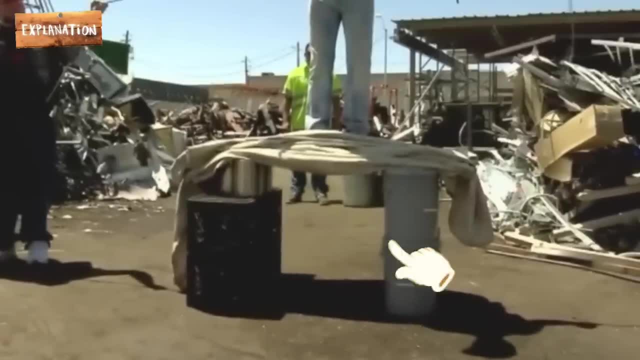 beside him had visible shadows. However, there is a camera cut when he climbs the slab. After the cut, we notice the angle of the shadow of the man in a fluorescent yellow shirt and the barrel next to him change. This happened because Criss positioned a mirror underneath the slab. 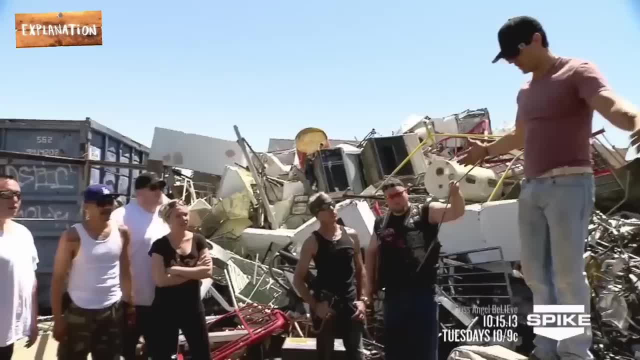 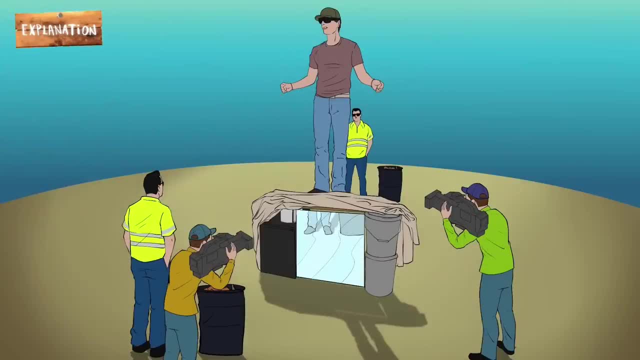 and between the two supports. Hence the camera cut was done so the magician could do a setup off camera. The mirror makes it impossible to see the objects behind him. As a result, he brings another man wearing a similar costume as the man behind him to the front of the mirror, Although the 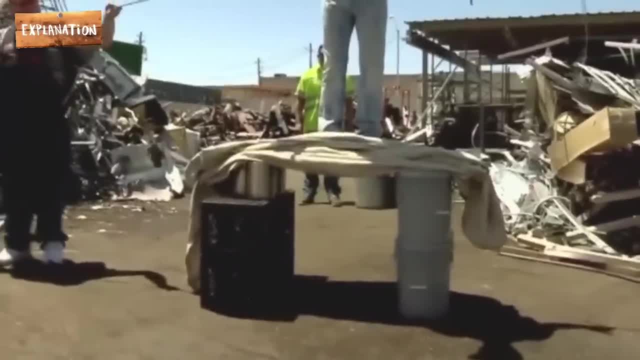 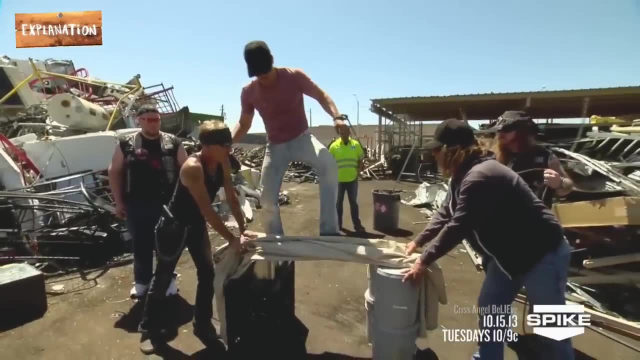 position of the camera made the reflections look like the man and barrel behind Criss. their shadows aren't the same as they were earlier. In addition, the color of the barrel before the camera cut and after the camera cut is not the same. Looking closely, we observe that. 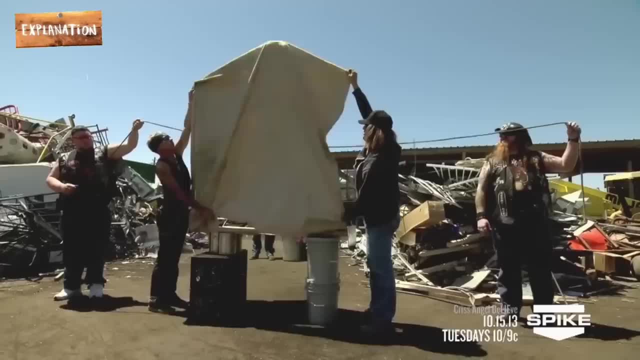 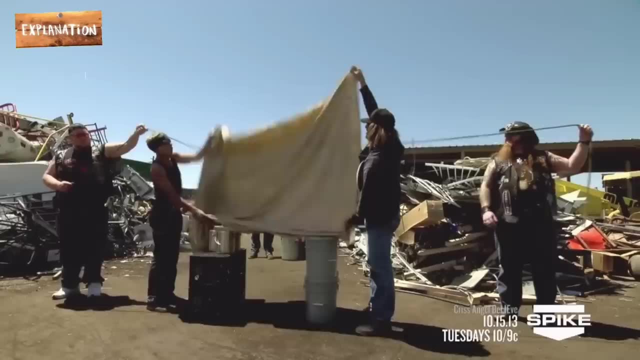 the shape of the ground after and before the camera cut was not the same either. When the magician's assistants dropped the curtain, he jumped off the slab and hid himself behind the mirror. Therefore, he used the mirror to trick the audience to believe him to be an invisible man. 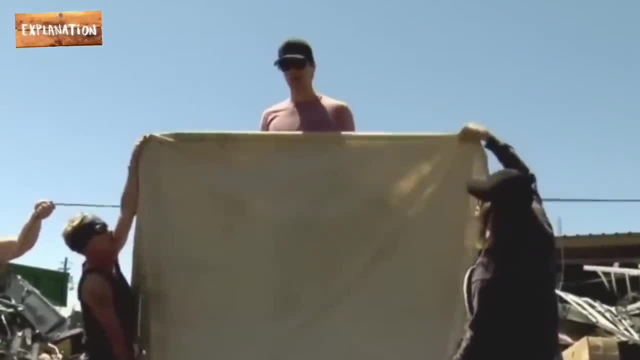 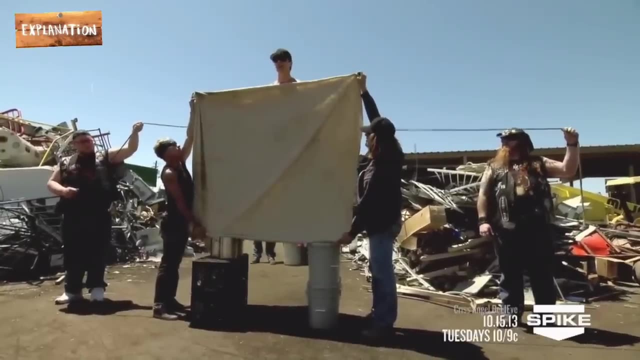 A moment before he disappears, we notice that he spent a few seconds talking to his assistants. During this moment, he cunningly unties his hands from the rope and ties them together, and his assistants were visibly loosening their grip on the ropes Due to his hands being free from the 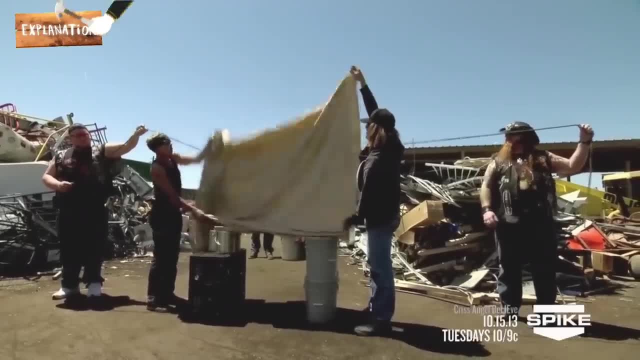 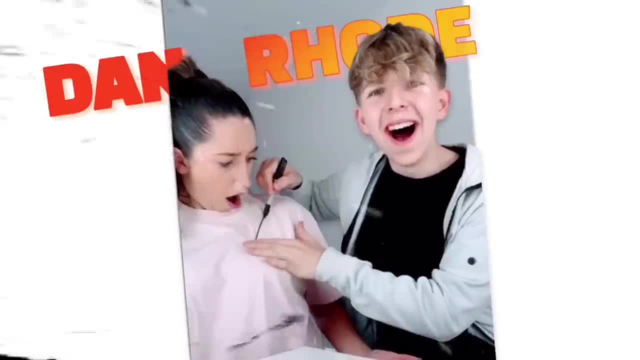 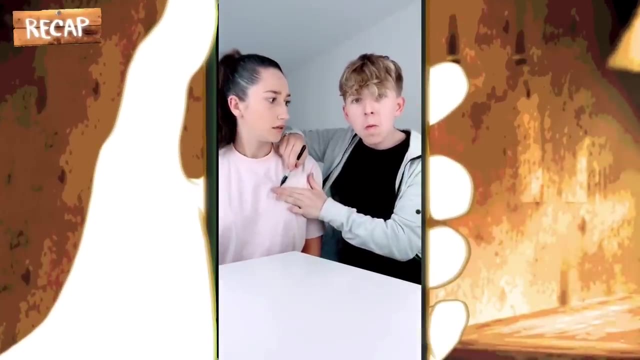 ropes. the magician visibly raises the curtain to conceal himself before jumping off the slab. Dan Rhodes' Viral Tricks. Let's do a quick recap of what happened in the performance. Dan's illusion begins with him drawing a line with a black marker pen on his assistant's t-shirt. 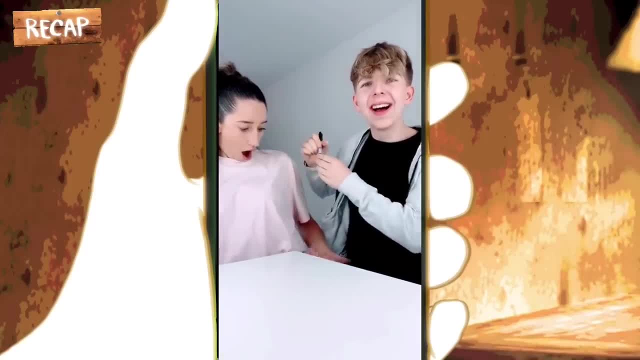 After which he starts to draw a line with a black marker pen on his assistant's t-shirt. Afterward he cleans the ink off her shirt magically with his bare hand. In his next trick, the magician puts the cap of the marker in his assistant's nose and makes it. 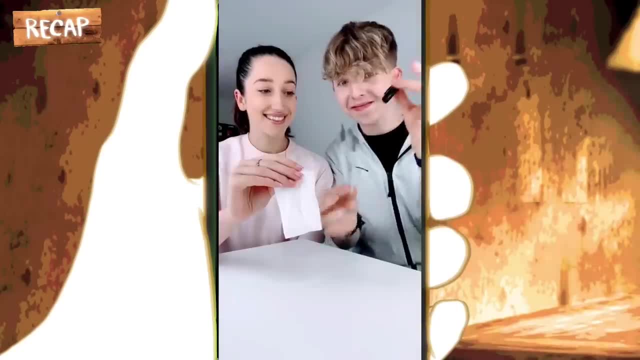 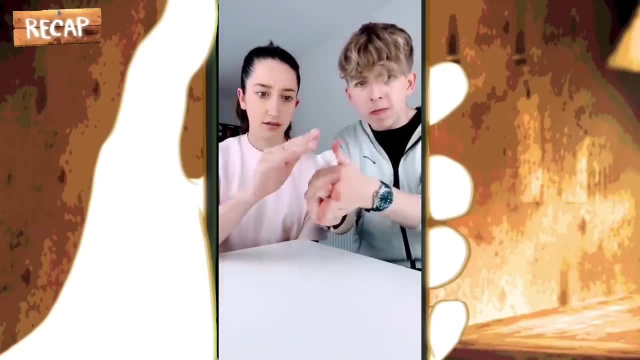 disappear into thin air. In Dan's last trick, he puts the pen between a folded piece of tissue paper while his assistant raises it. Then he mashes it together by clapping his hands and the marker vanishes out of sight. How did he perform his tricks? Here is how he executed them. 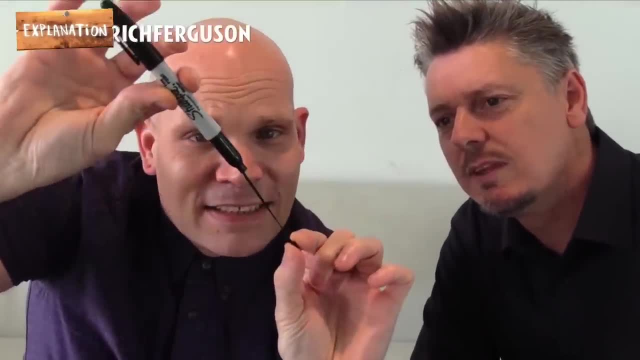 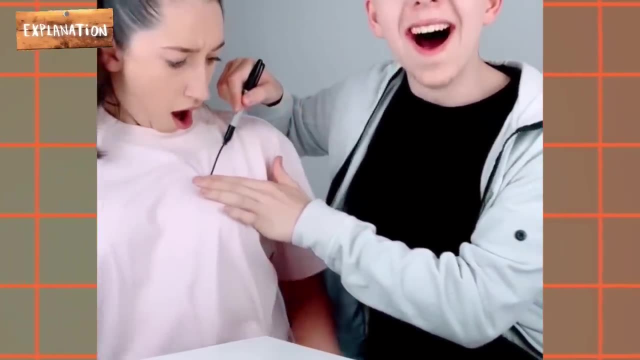 The tip of the black pen isn't a real tip but a black stretchy string. To make the trick work, the magician presses the tip of the marker with his finger on his assistant's shirt after writing on it. Thereafter he lets go of the tip and the tip gets pulled back. 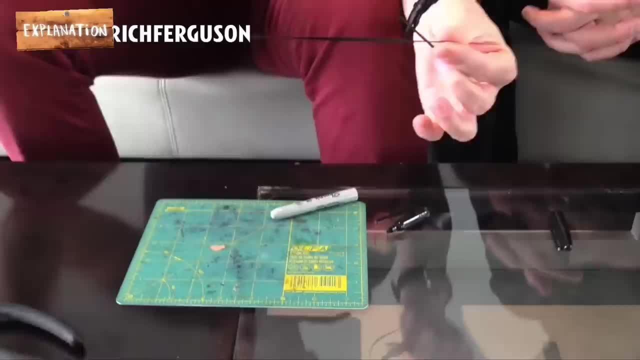 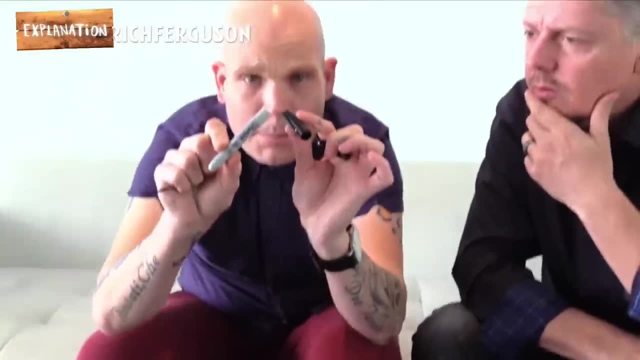 into the pen due to the elastic nature of the string. He got a flat elastic that is approximately 7 inches long and ties a knot four times at its tip. Afterwards he dismantles a real pen, gets rid of its ink and pulls out its nib using pliers. Once he removes its nib, 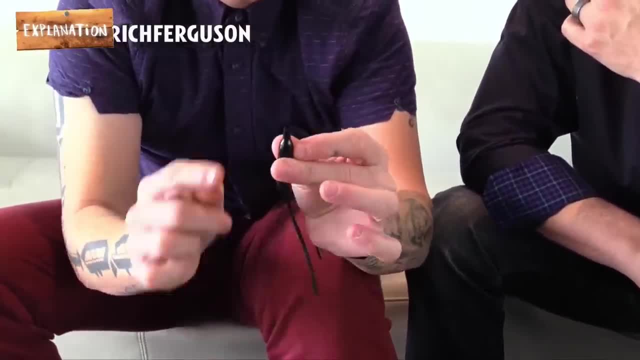 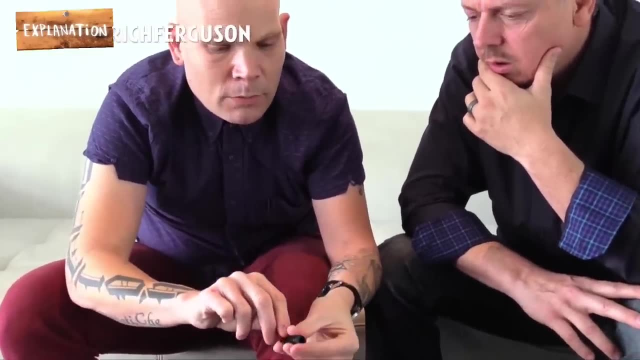 he passes the knotted flat elastic through the upper part of the pen. The knot ends up at the tip of the upper part of the marker where the nib was positioned. Thereafter he pulls the elastic over the upper part of the pen and presses it with his thumb. 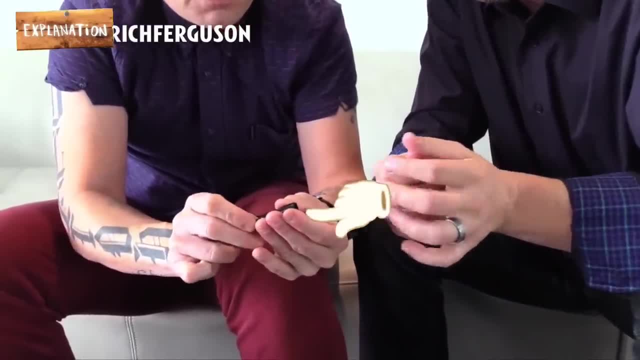 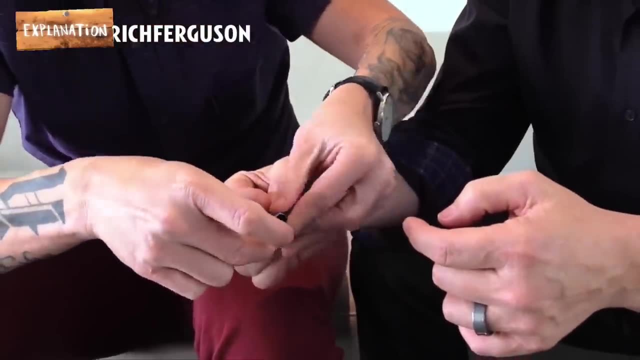 However, he ensures that he doesn't pull the elastic too hard, but enough to suck up its slack so it can be extendable during his trick. Once he sets up the elastic, he tapes the part his thumb is pressing on the upper part of the pen. Then he fixes it into the marker's lower part. 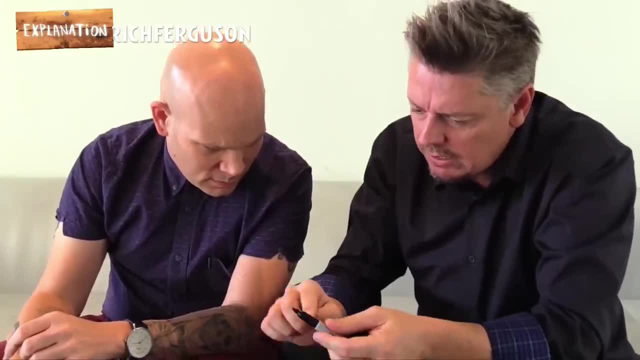 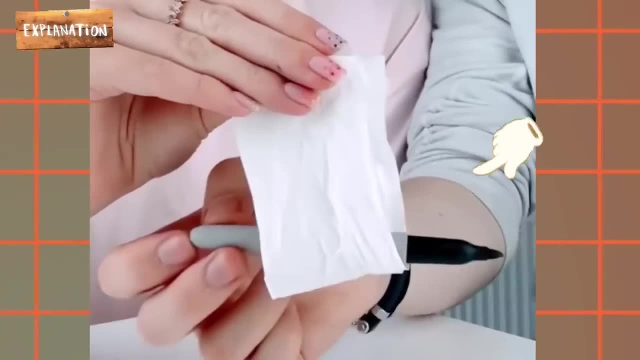 concealing the tape and cuts off the excess part of the elastic hanging outside the tape. The second trick, where he puts the marker in between a folded tissue paper. it isn't made of a solid material like real pens. Instead it is made of flimsy rubber material and, as a result, 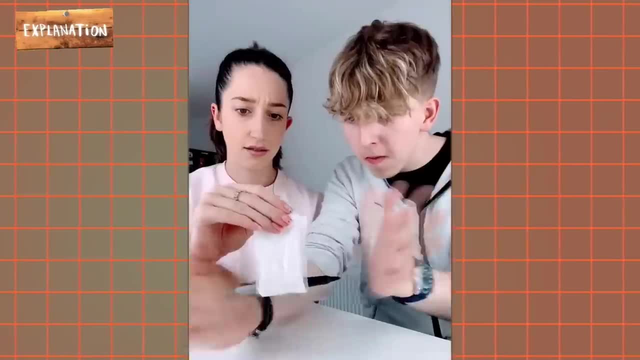 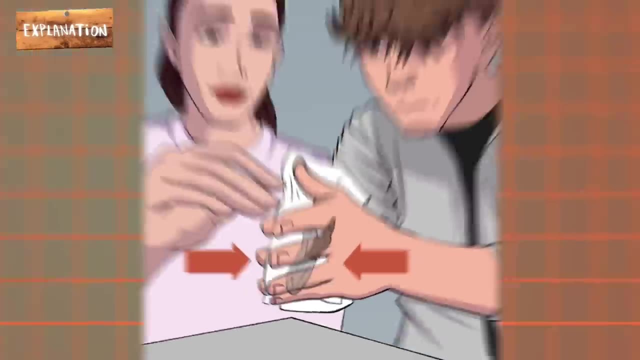 it wasn't as straight as a real marker would be. Hence, when he claps them together, the pen vanishes. Once the magician claps his hands, he crushes the rubber and it squeezes up just as a loaf of bread would. Hence the marker didn't disappear into thin air, but he folded it up in. 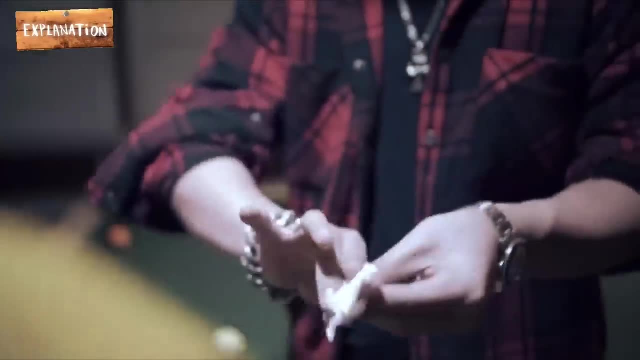 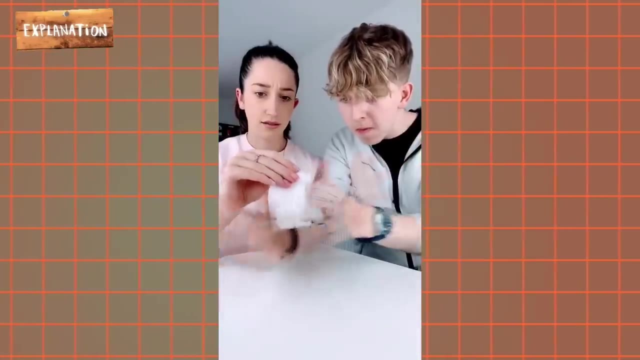 the tissue using the sans-mines vanishing sharpie trick. We notice that there is a camera cut after he squeezes the marker and tissue paper. He did this to get rid of the mashed-up pen, so it won't be obvious that it was still in the tissue after. 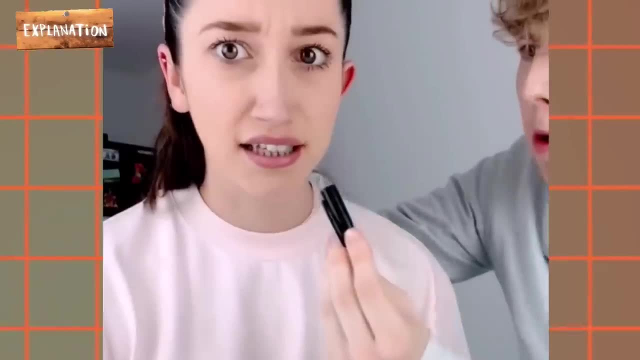 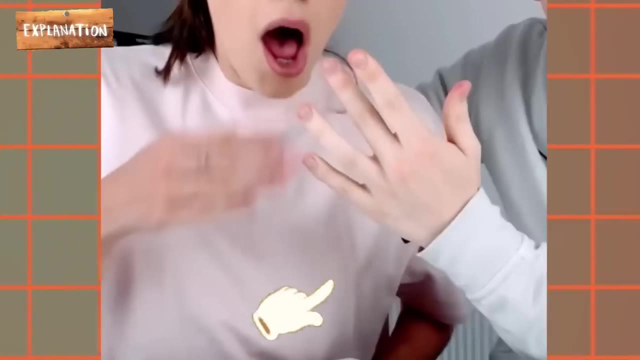 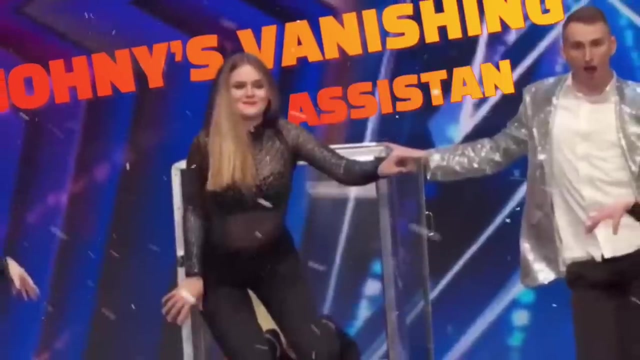 he squeezes it. An elastic thread is attached to the cap and he attempted to pull it into his sleeve, but he couldn't pull the move off perfectly. Looking closely, we observed it in his hand in the form of a little bump when he tried to pull it into his sleeve. Johnny's vanishing and appearing. 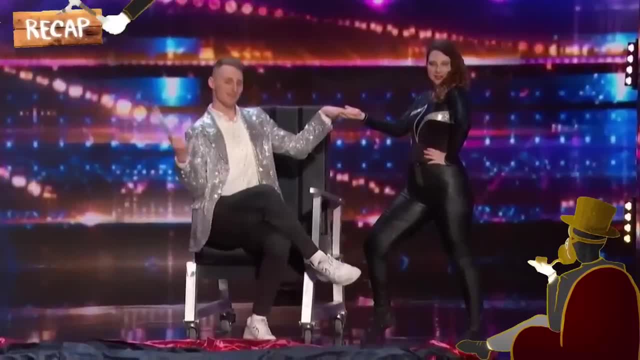 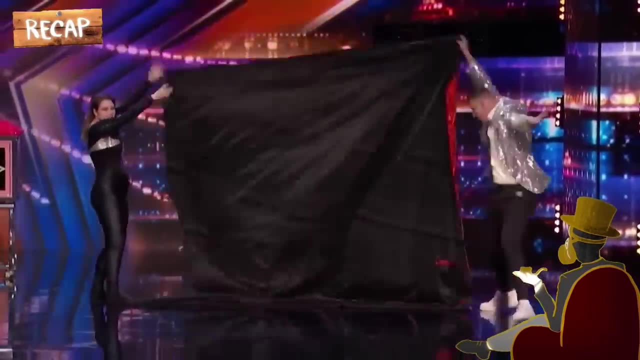 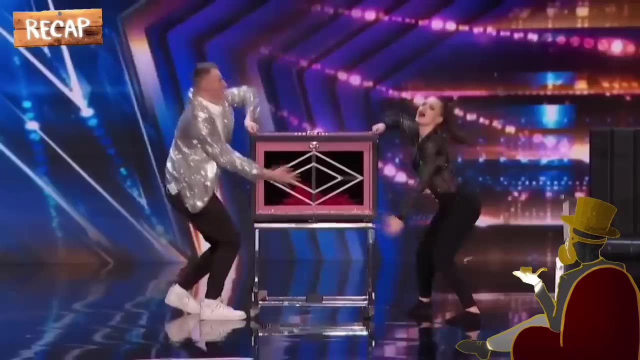 assistance. Let's do a quick recap of what happened In the performance. the magician begins his illusion by sitting before a box. Once he stands up, he raises a curtain with the help of his assistant and a woman appears on the chair. when the curtain is dropped, Then he puts a pink neck muffler in a see-through box and closes it. When 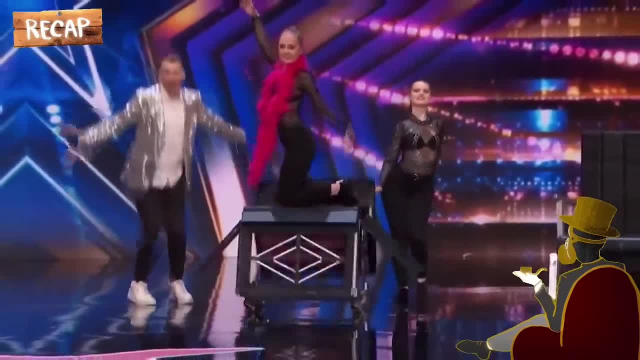 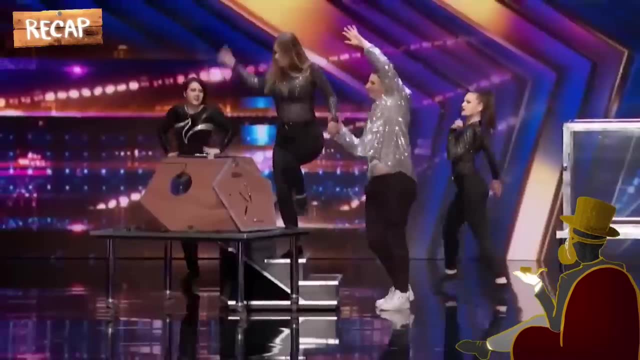 he opens it, another woman appears wearing the muffler around her neck. Afterward he covers an empty glass box with a curtain, but when he drops the curtain, another woman appears in the box. After that trick, his assistant enters another box that isn't transparent like the previous boxes. 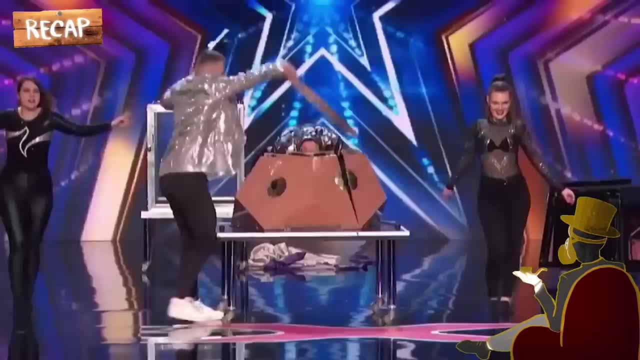 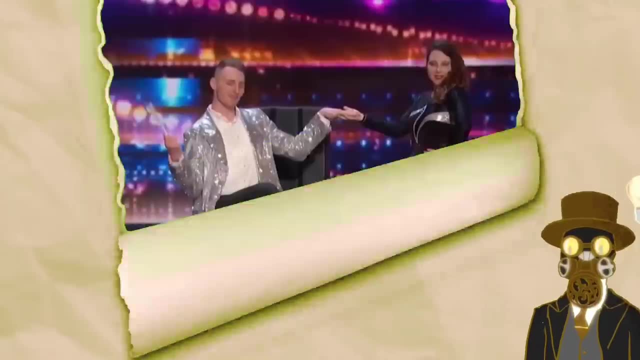 and closes it at the top. He moves the box to another position, opens it and a man appears out of the box Wondering how he did his tricks. Here is an explanation. Although the back of the stand was empty before Yannick sits on the chair, he tricks the audience into believing that he. 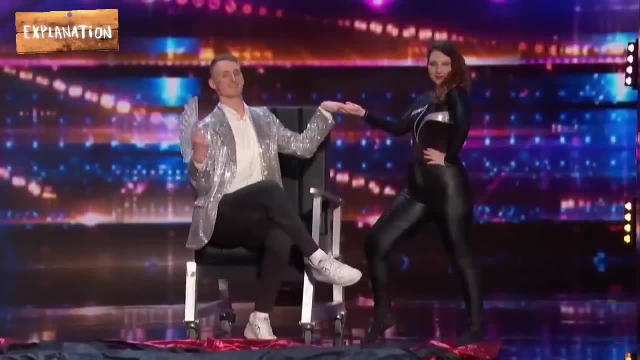 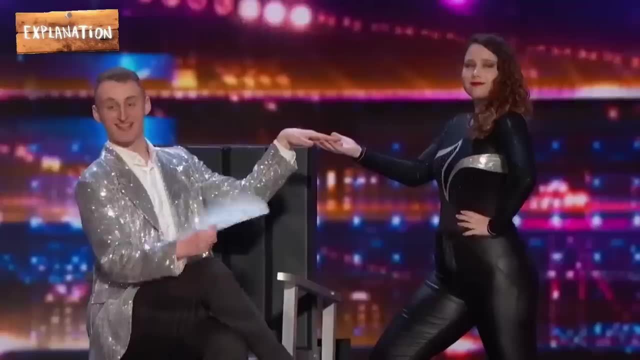 mysteriously made the woman appear When the magician sits on the chair and holds his assistant's hand. the woman that seems to appear after they drop the curtain is crouching. She was in a crouching position behind the stand where Yannick is resting his back when he sits on the chair. 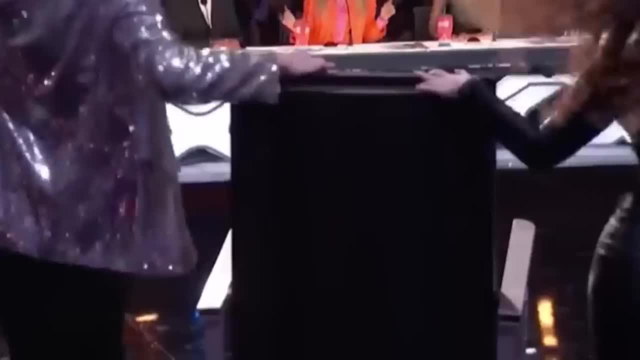 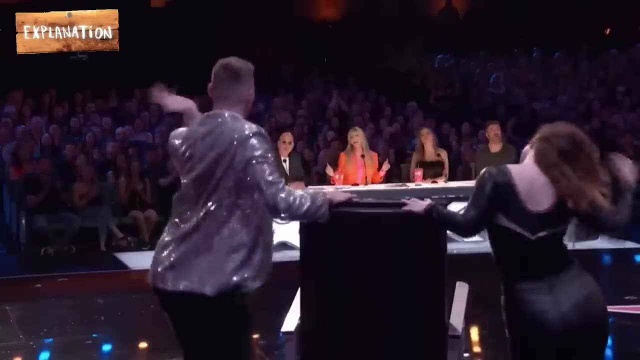 After the camera is focused on the audience and brought behind the stand, she can't be seen in her crouching position. However, she remained in her crouching position and was covered with a cloth when the camera was brought behind. Furthermore, we observe that when the camera was brought behind, 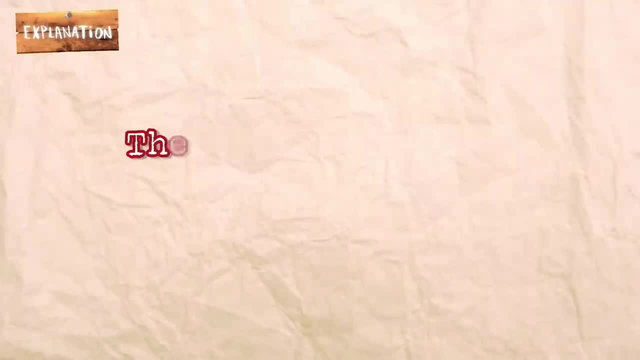 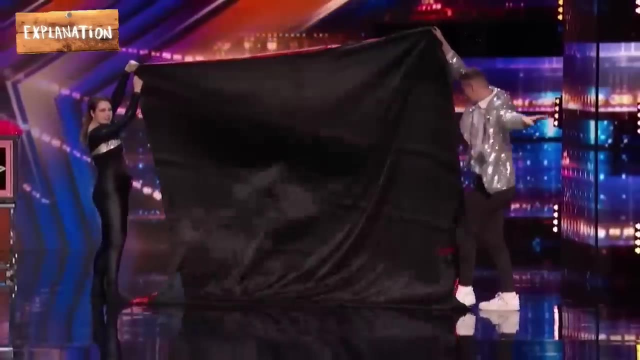 the stand. it didn't show the base of the stand. The base was cut off from the camera's view to prevent viewers from noticing the crouching woman covered with a piece of cloth. So when the magician and his assistant raise the curtain, she jumps forward and sits on the chair. 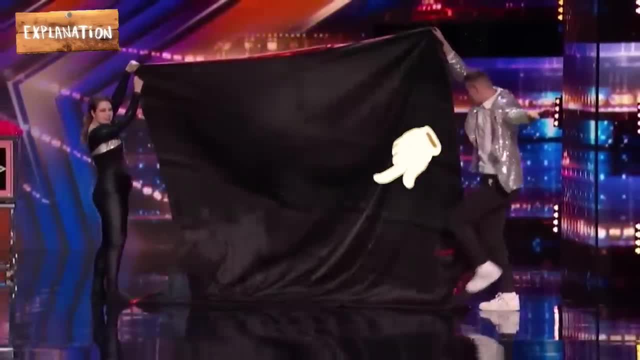 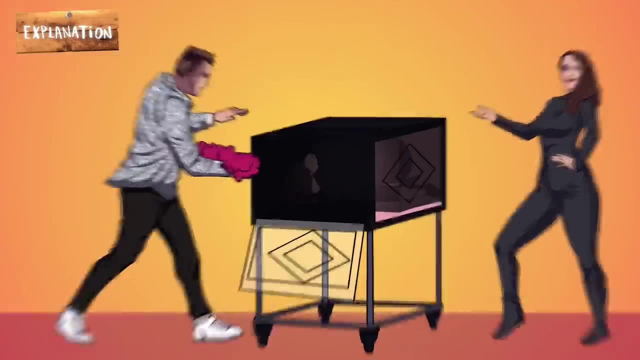 Closely, a slight bump can be seen on the curtain when she jumps forward to sit on the chair. In his subsequent illusion, where he puts the neck muffler in the see-through box, the woman was crouched in the box. The box has a small section at the front of a larger section. 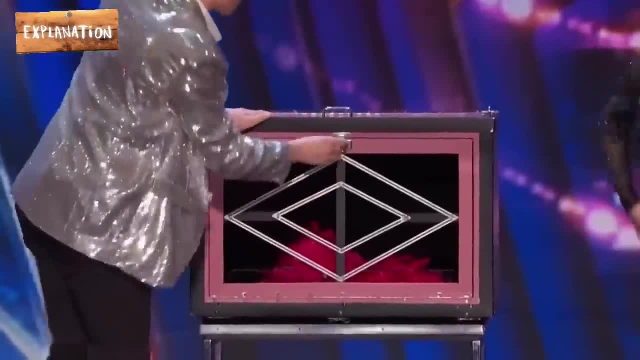 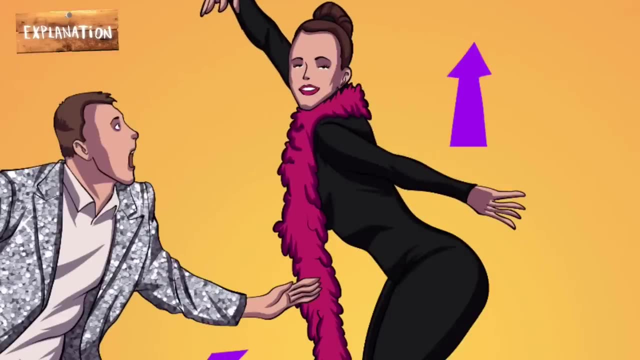 where the woman is crouched. When Johnny puts the pink muffler in the small section, he closes the box and opens it. Although it seems like the woman suddenly wears the muffler around her neck when he opens the box, she had another muffler around her neck. When Yannick opens the 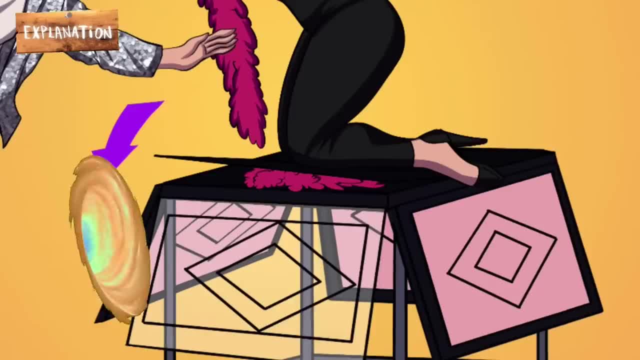 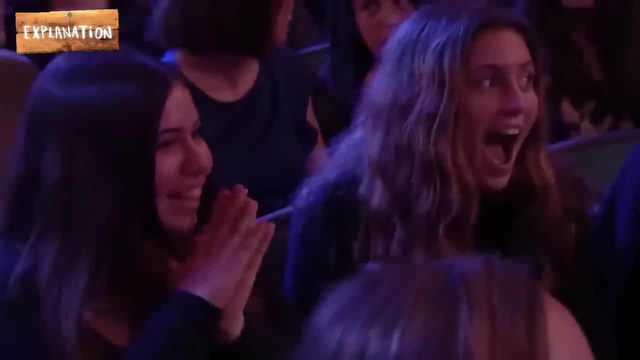 box and reveals the woman. The slab demarcating the two sections in the box falls to the front. As it falls to the front, it covers the muffler Johnny put in the small section, making the audience believe it's the same pink muffler. In his third trick, where he uses a glass box, we initially observe that the 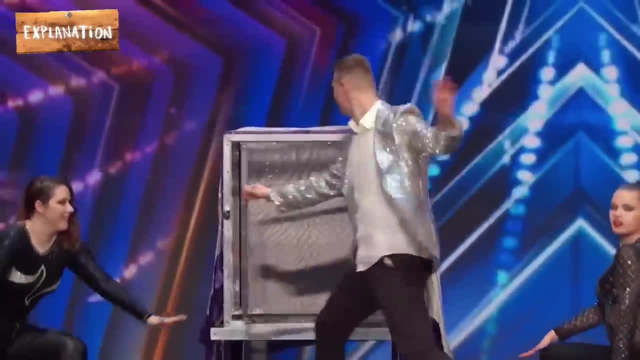 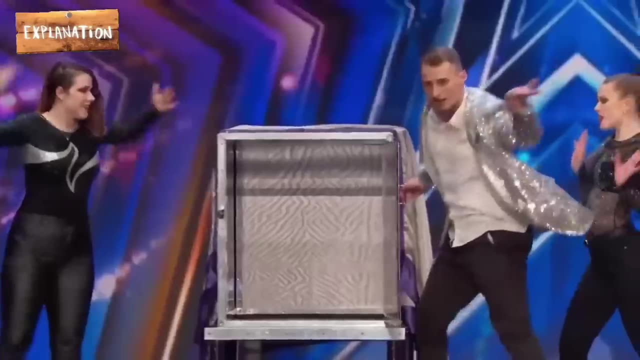 box has a metallic backside, But when the woman appears after he closes the box, covers it with a curtain and removes the curtain, the backside changes to glass. The metallic wall that seemed to be at the back of the box is similar to the demarcation slab he used for the box in his 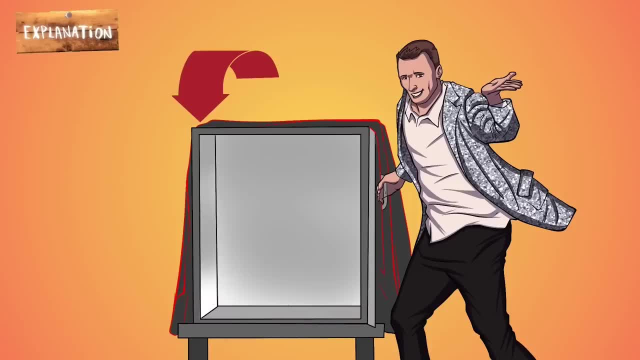 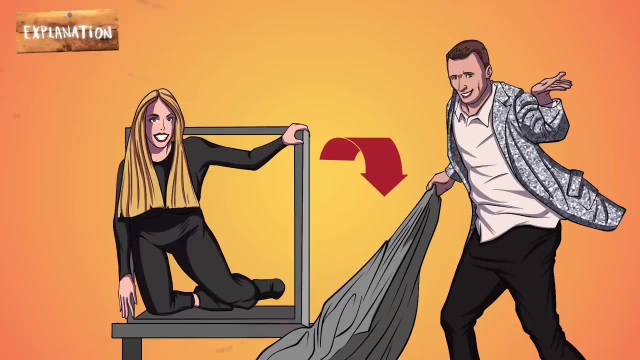 previous trick. As such, the metallic slab demarcated the larger section where the woman was crouched from a small section in the front. Once the magician opens the box to reveal the woman, the metallic slab falls to the front and makes it seem like the woman appears mysteriously. 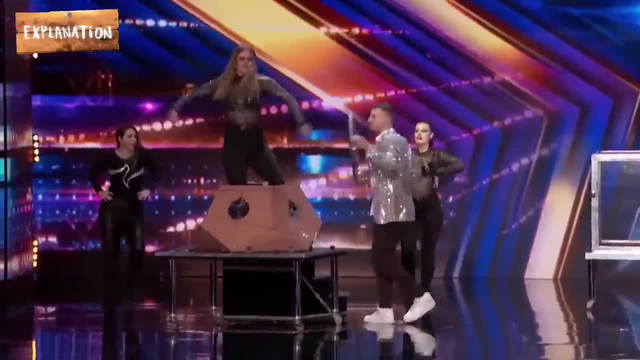 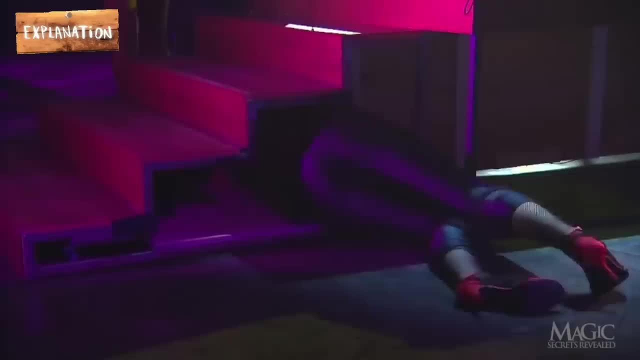 The magician's final illusion where a woman enters a small box placed on a stand, already had a man in it before the trick began. Instead of entering the box, the woman went behind the box and into a removable staircase through a hole in the stand. Afterward, Yannick moves the. 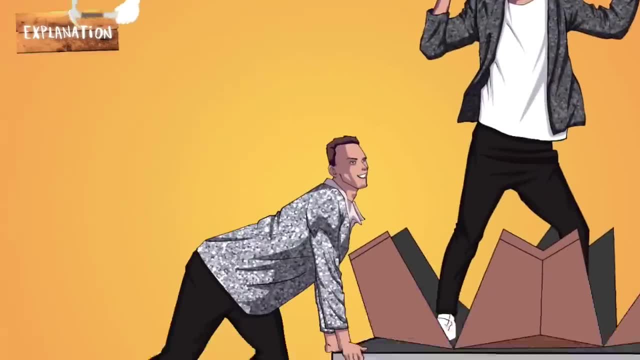 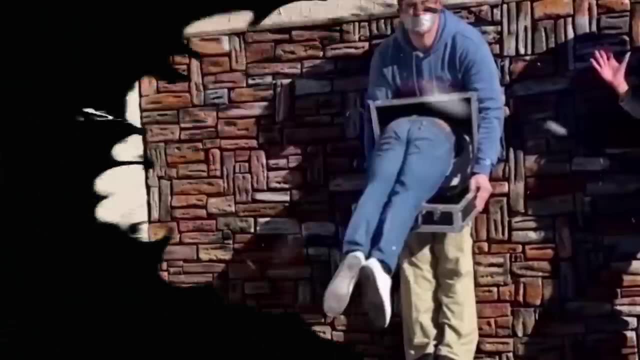 stand and opens the box. When the woman enters the box, the woman goes behind the box and into a stand with the box to another position and reveals the man in the box, while the woman remains in the staircase. Xavier's suitcase teleportation trick. Let's do a quick recap of what happened in the 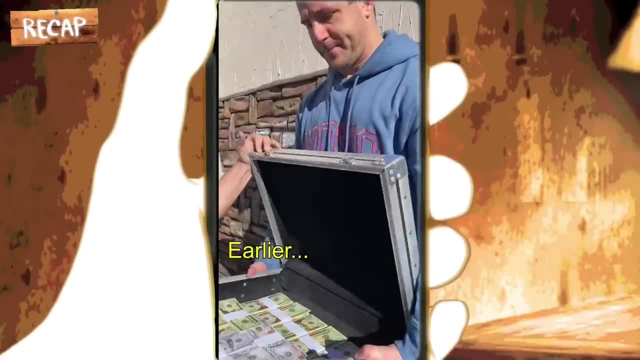 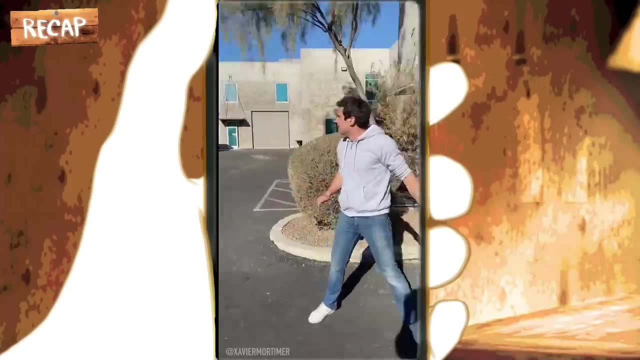 performance. Xavier's illusion begins with him and his assistants placing an open briefcase in a man's hands, cuffing his wrist to the box and taping his mouth. After taunting a police officer, he jumps into the briefcase and is nowhere to be found Thereafter. 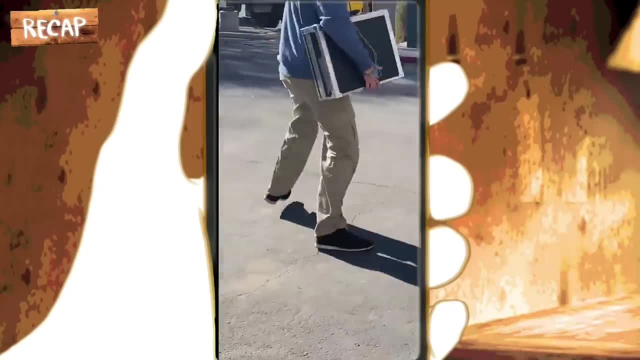 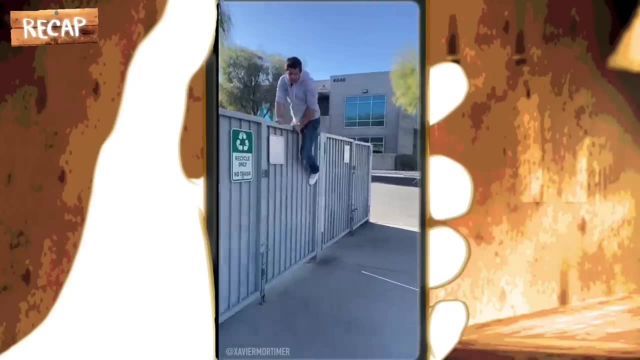 his assistants remove the tape from the man's mouth, close the briefcase, uncuff the man's wrist and throw the briefcase over a fence. Incredibly, the magician comes out of the briefcase, jumps over the fence and flees from the scene. How did he execute his tricks? Here is an 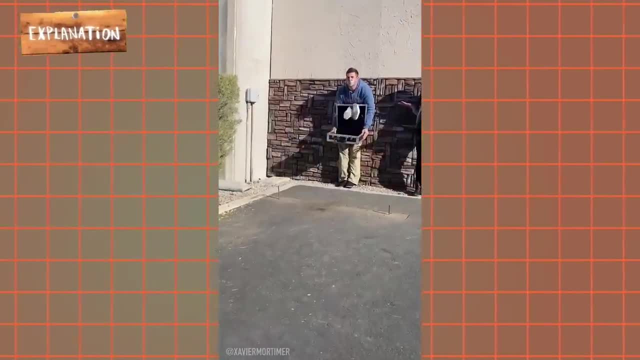 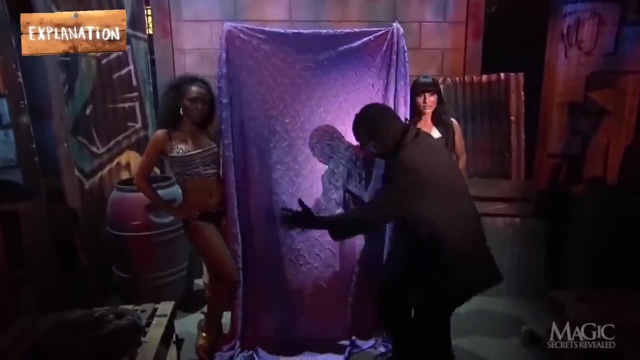 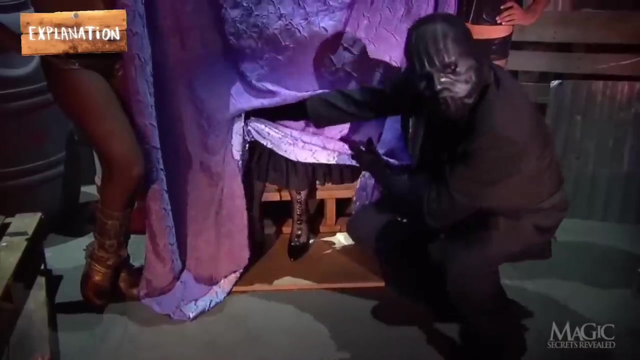 explanation, We will compare the trick Xavier performs in this clip to a similar classic stomach removal illusion executed by a masked magician. In the masked magician's trick, a curtain was placed above a girl's head and used to cover her in her entire body. He lifts the curtain to show the audience that she's still behind the curtain by. 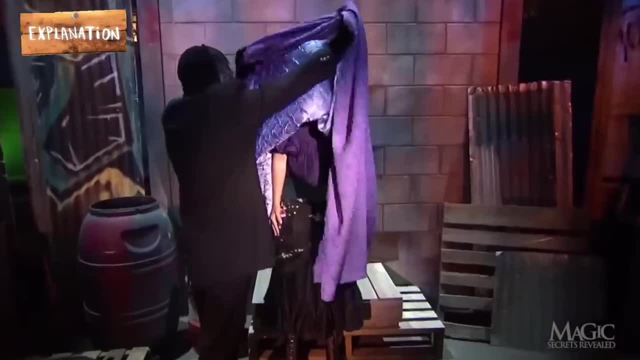 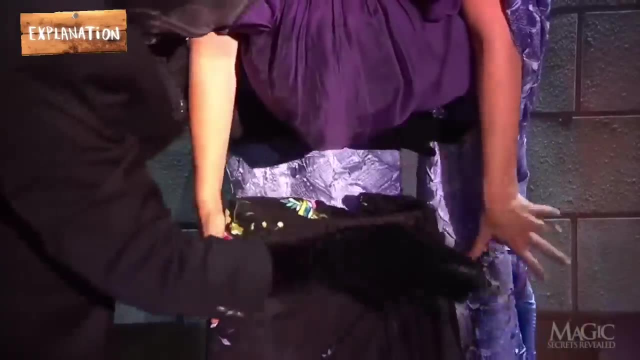 showing just her legs. However, when the magician lifts the curtain, the girl's main section isn't visible and her upper body appears to be detached from her lower body. He puts his hands through the space between her upper and lower body, and his hands go through without any hindrances. Also, 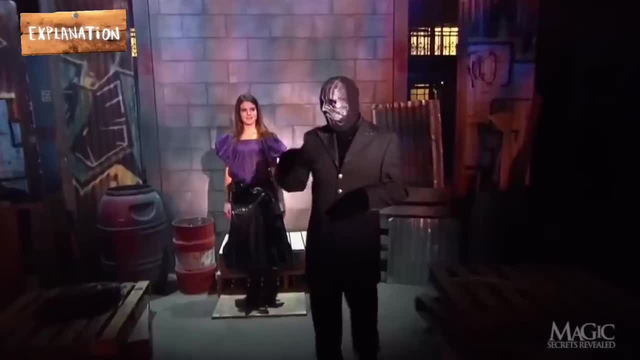 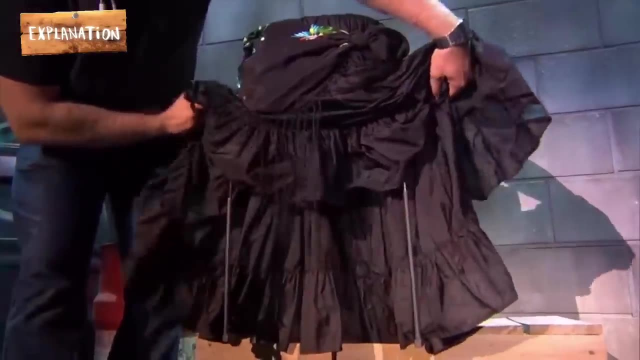 the girl didn't seem to be bleeding or in any form of discomfort. At the beginning of the illusion, the girl remained in a particular position without moving her legs. It turns out she didn't wear the skirt she seemed to have on throughout the illusion, and 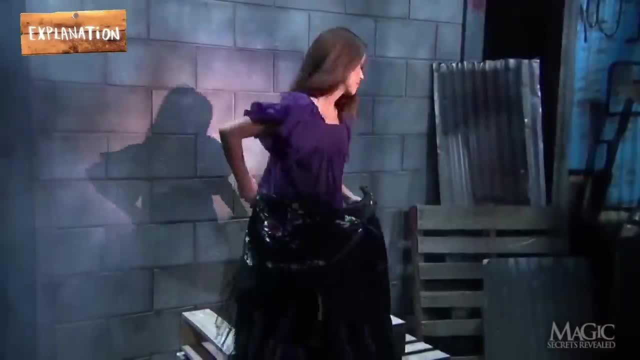 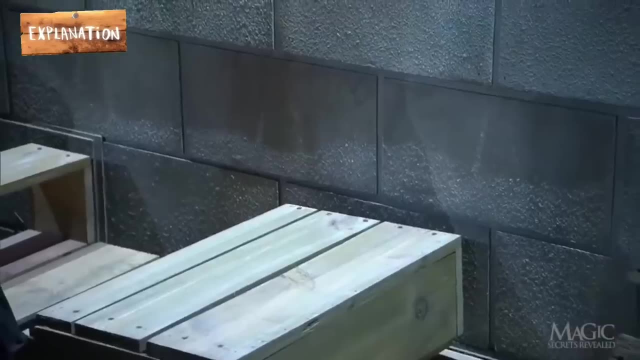 it is held in place by a wire frame. When the curtain is raised, she sneaks through the back of the skirt and bends down behind the skirt. Also, the wall behind her has a false panel which is removed by a man behind the wall and she lies back unseen Afterward. a matching panel that has 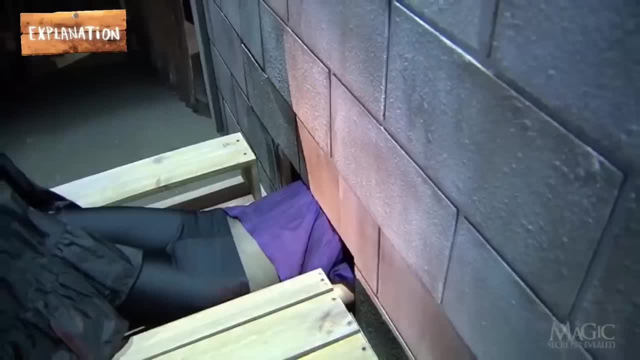 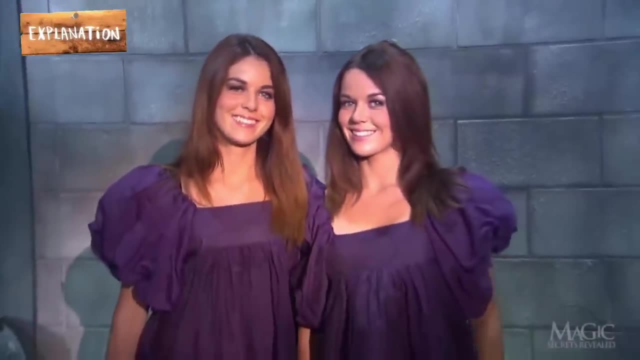 a little dissection, for her body was placed in the position of the false panel. This enables her legs to be seen by the audience, while her body is unseen. As it turns out, the masked magician employed a set of identical twins. Before he begins his illusion, the second girl is. 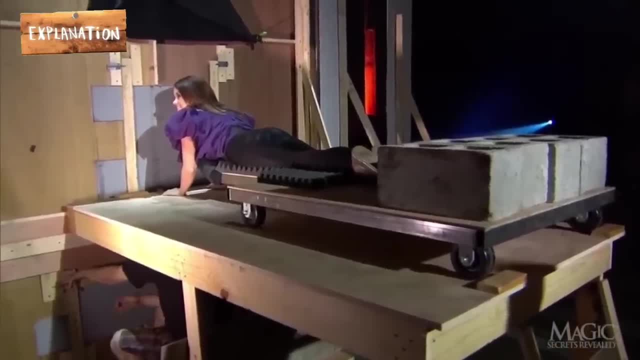 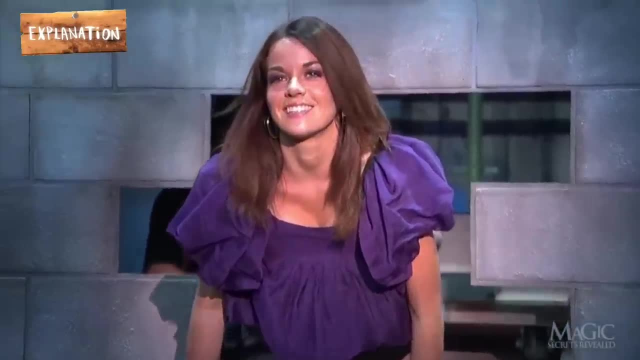 positioned on a rolling platform balanced with cinder blocks behind the wall. The magician assistants remove the false panel on the upper part of the wall to slide out the rolling platform with the other twin on it. Once the girl is slid into position and aligns with the skirt and her 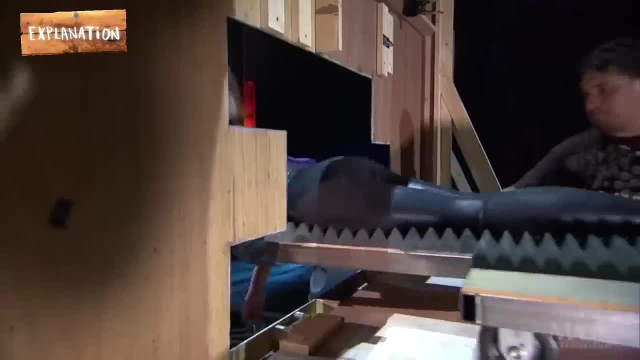 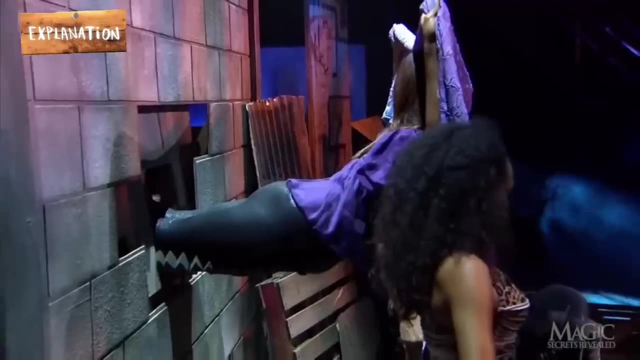 sister's legs. the curtain is placed on her head, With the cinder blocks placed at the other end of the rolling platform behind the wall. the girl is prevented from tipping over To conceal the hole, another false panel is fixed to the wall. In addition, we notice the girl's strange posture. 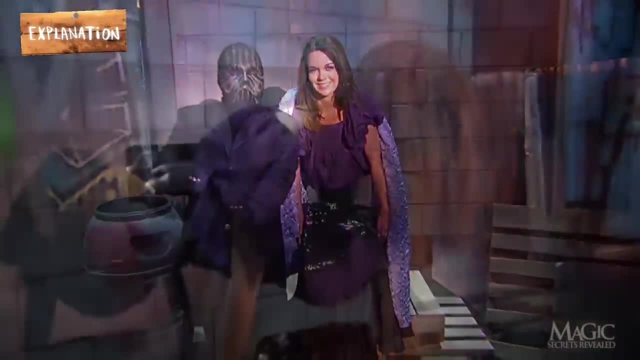 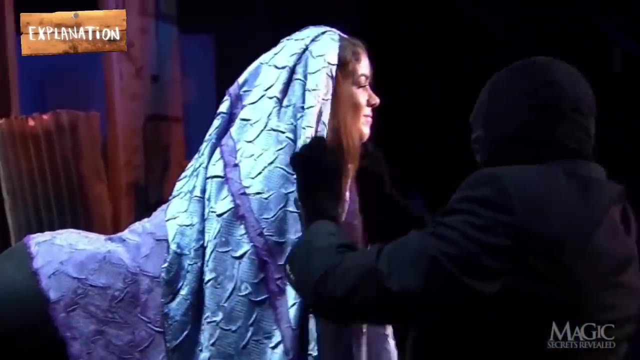 when the curtain is removed. This is because she has to lift her head and upper body awkwardly to make it seem like she is standing. The magician sets up the curtain carefully above the head and shoulders of the girl on top to hide her uncomfortable stance. Additionally, her bulky